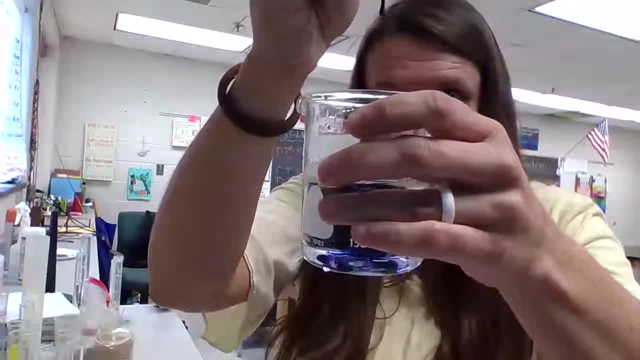 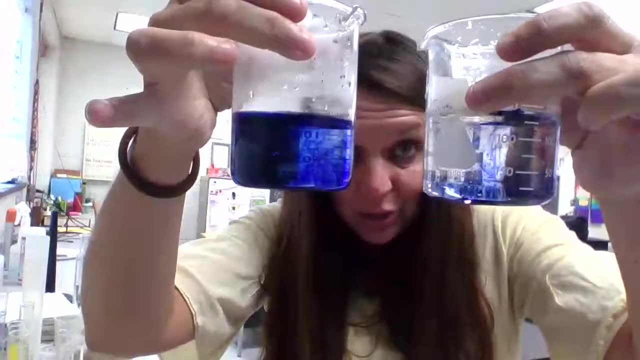 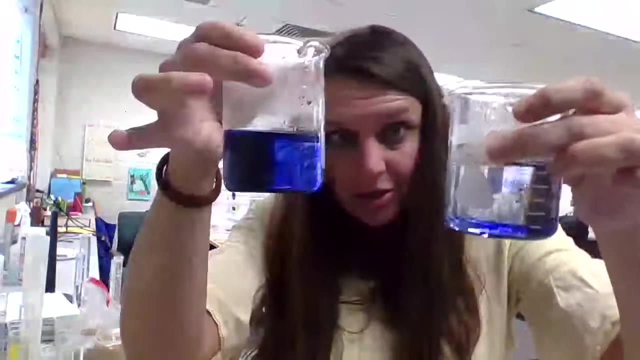 Three, four, five. Now if we notice we had a lot more particles moving around in the warm water than we did in the cool water, Kind of see that It also spreads around much quicker in the warm water than it did in the cool. So that's our big observation, So our main. 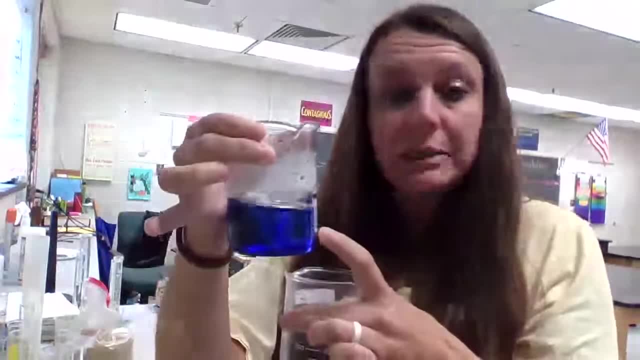 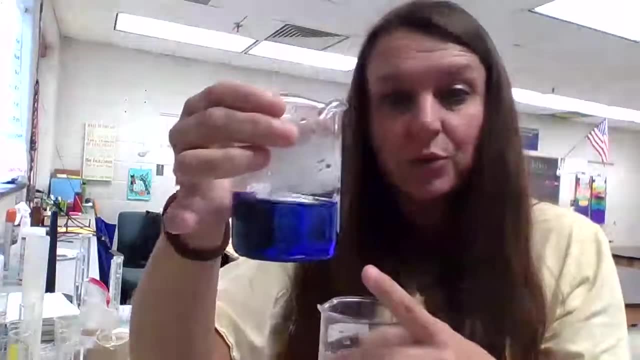 thing that we want to see here is that temperature is really making a difference with our particle motion here. The warmer the water, the faster those food coloring particles kind of move around and spread out. The cooler the water, the longer it's taking. 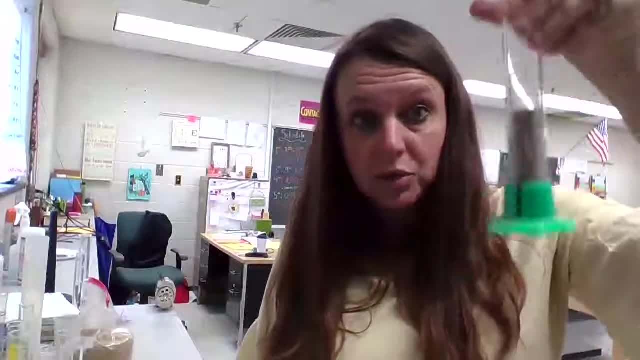 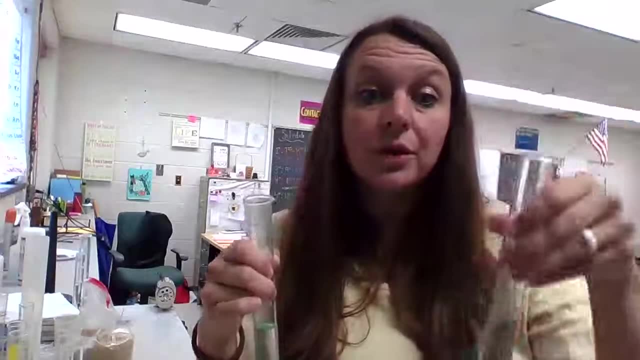 So the next demo is with 25 milliliters of sand and 25 milliliters of water. So what we want to do is we're going to add this water to the 25 milliliters of sand and we're going to see what. 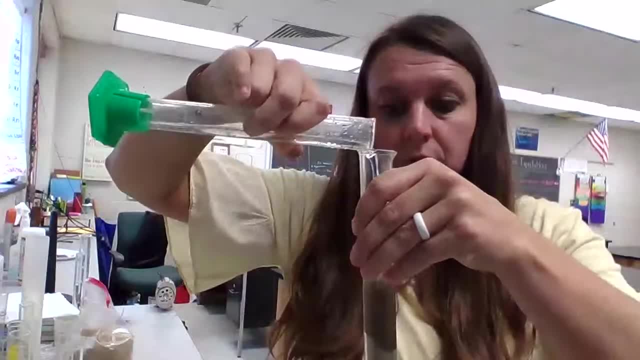 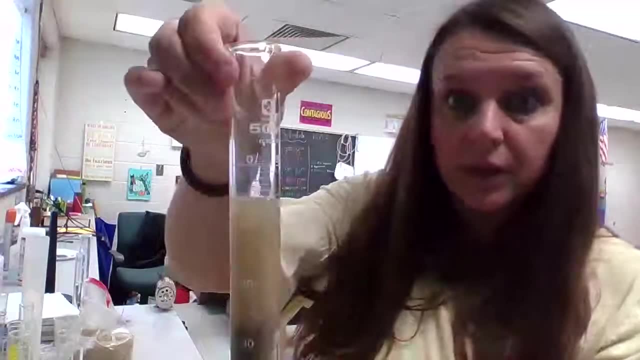 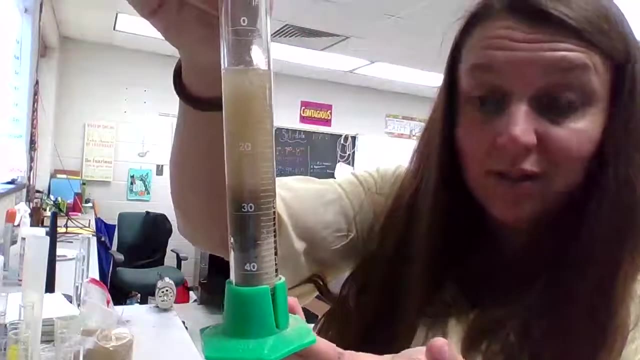 happens. So you would think 25 plus 25 is 50, right, So it should have been up around the 50 milliliter mark. But what do we think is happening here? That water is filtering through some of these sand, So sand is like our particles, right? 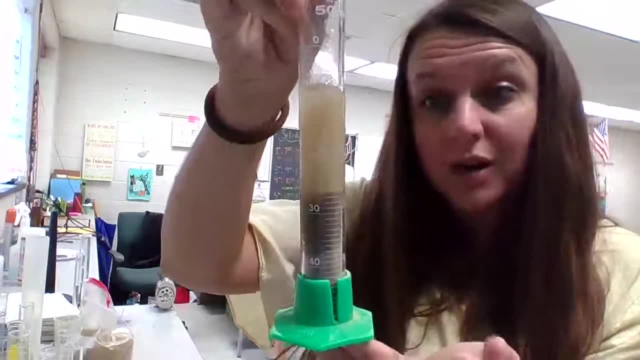 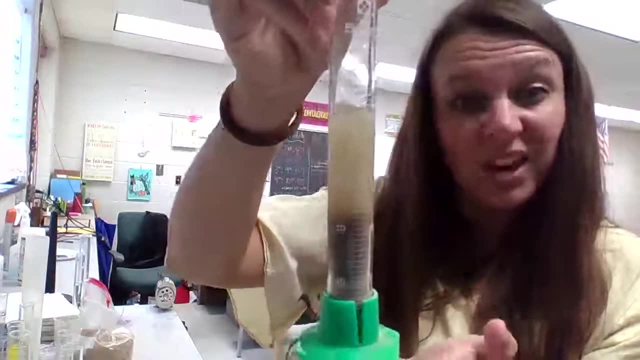 And there are spaces in between our particles, So that water is filling up some of the space that's in between our sand particles. Yep, Kind of cool And it'll keep going. Eventually it'll settle. It'll be all the way like kind of down here once it's all done, But this: 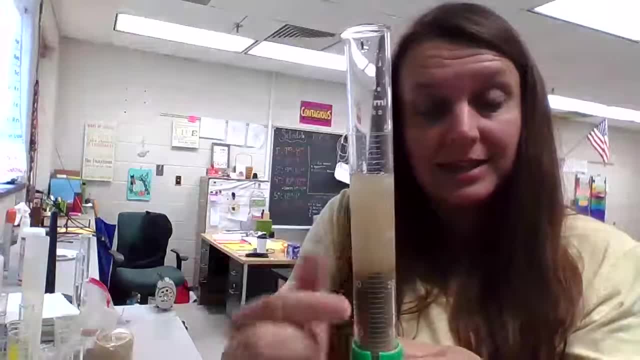 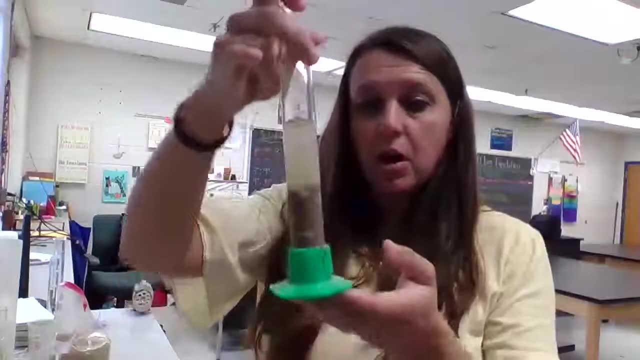 is all about the water filling in that space. So we're going to add this water to the 50 milliliter mark. So that's the space that's in between those particles. So our sand activity also shows us that sand is kind of its own unique particle and water. 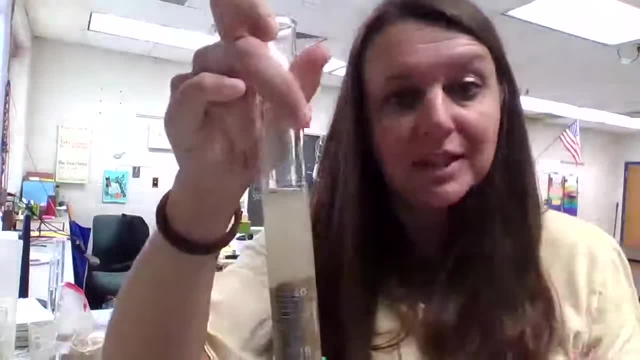 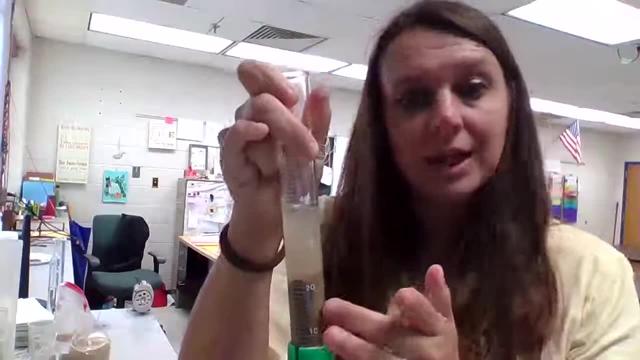 itself is also its own, different one. They don't just automatically mix together and make a new particle. They don't come together and just make mud right. They're still having their unique properties of sand as being one particle and water as another. 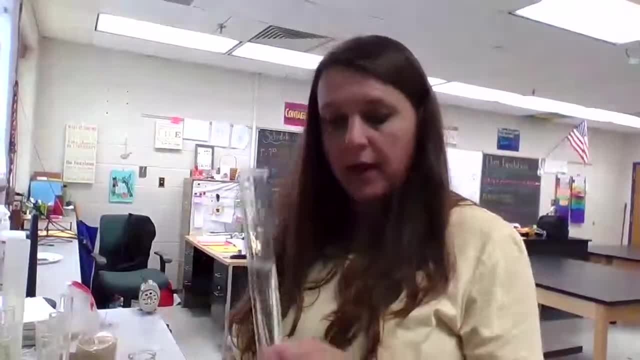 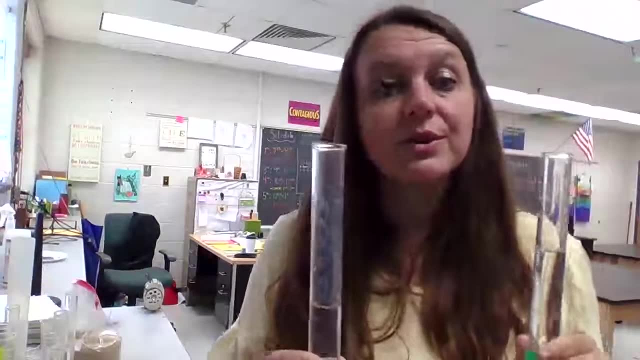 Okay, All right, In our next demo we have, We have 40 milliliters of alcohol and 50 milliliters of water, And what we're going to do is we are going to mix the alcohol and the water And part of your, One of your- 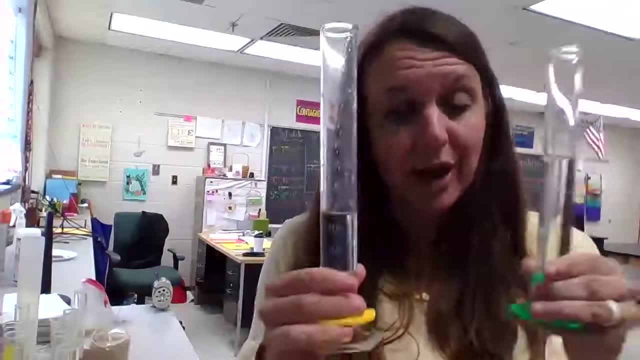 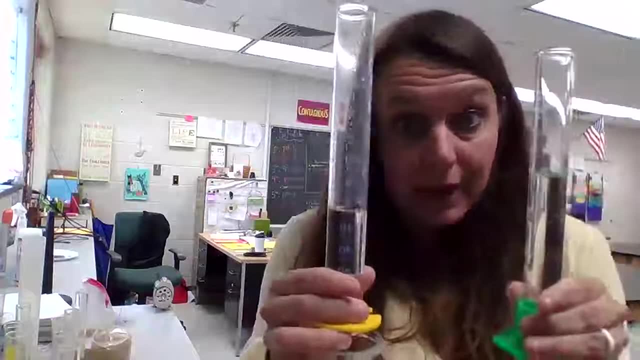 questions in your sheet asks you to make a prediction about how much you think we'll have when we mix the two together. So if you haven't done that yet, go ahead and do it. So hit, pause and take your guess. And we're going to go ahead and mix them, So pause if 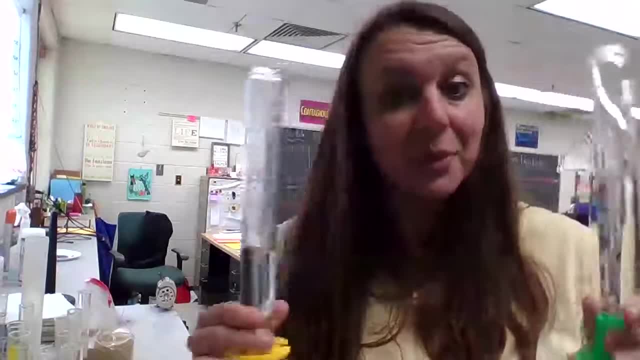 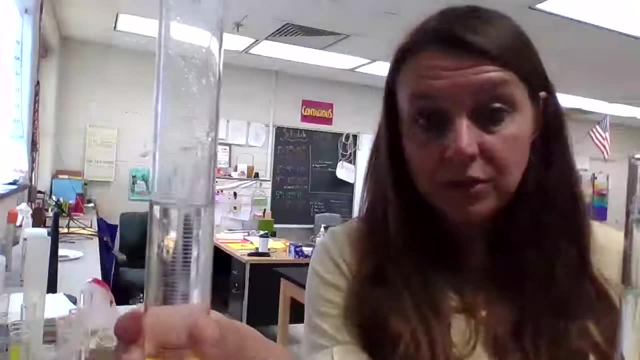 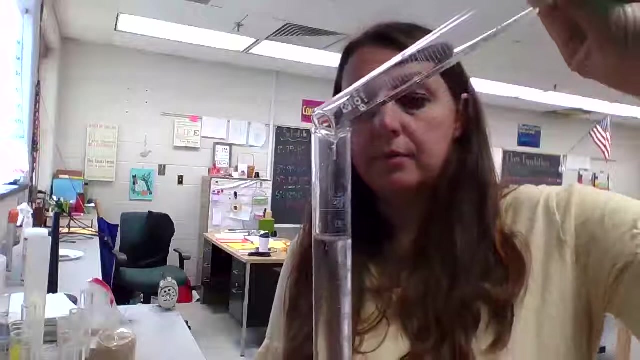 you haven't taken your guess. All right, Welcome back. Thank you, I paused and you're coming back to the video, All right, So I'm going to pour in my 40 milliliters into my 50 milliliters of water, with my alcohol going into the water. So it should have been. 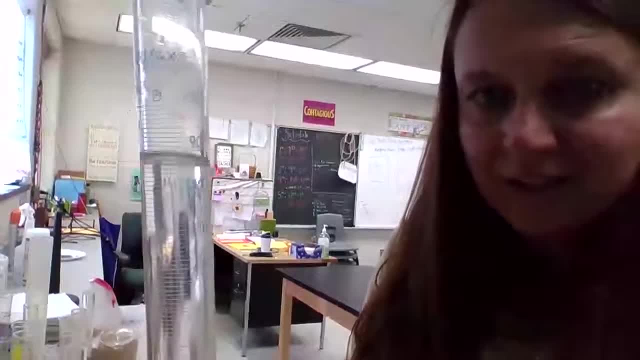 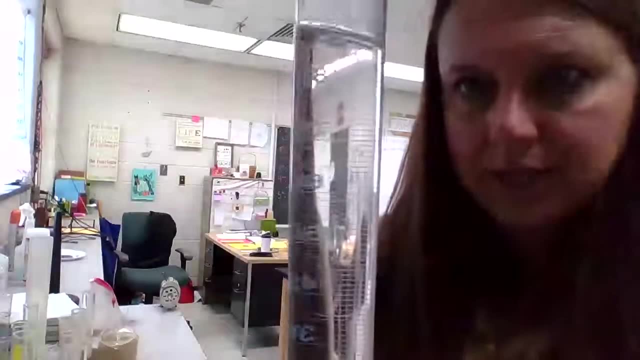 right about 90, right. However, we didn't really get there. We're not all the way at 90. So that's kind of a strange thing, And it's also- I don't know if you all can see it- 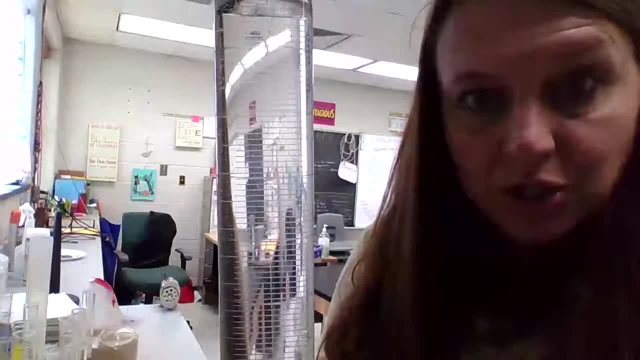 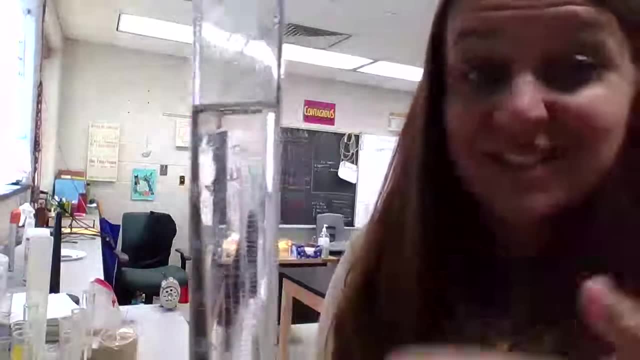 But if you look the little particles, there's little bubbles that are just moving all over the place, these little air bubbles. So what that is showing us is that particles are always in motion, These things are always moving back and forth. It also shows us that there 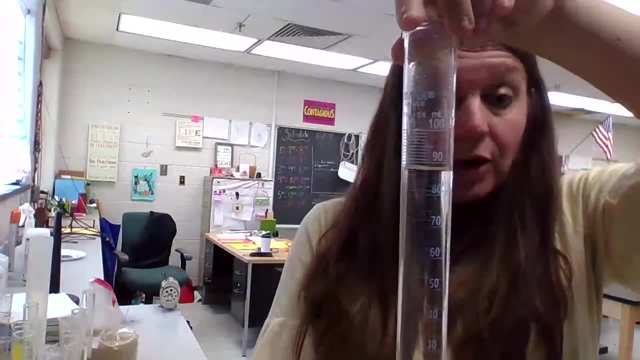 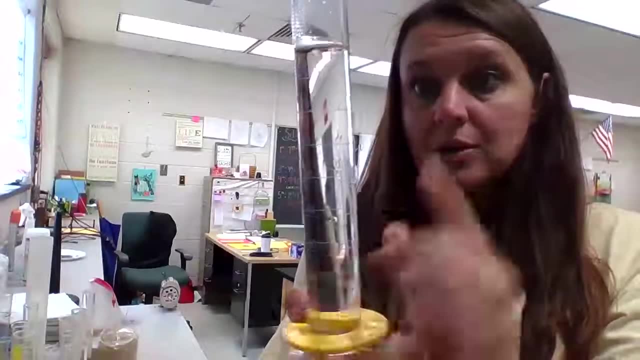 are space in between these particles, that some of the alcohol is kind of mixed in, and there's spaces in between each where they're kind of combining, flowing against each other, Also showing that there is still movement with these particles all the time. All right, 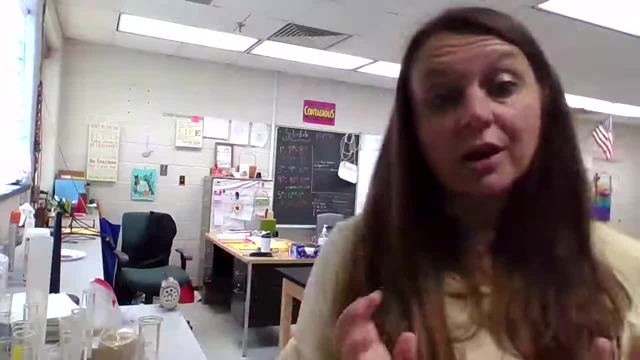 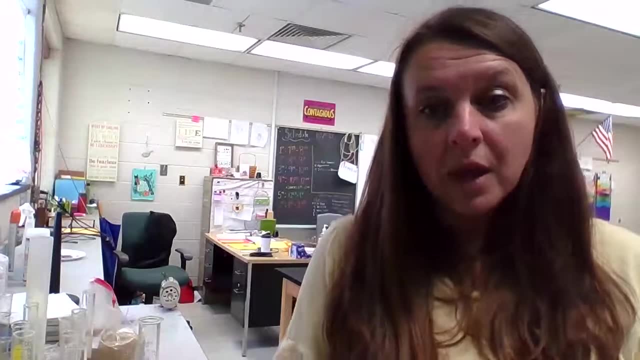 So make sure that you all are still filling out that sheet. There's a little chart at the bottom that I'd like you to think about, which demo showed each of the particle theories of matter. You can have more than one answer for each section, So that's kind of what I want you to think about- And yeah, that was our demo.